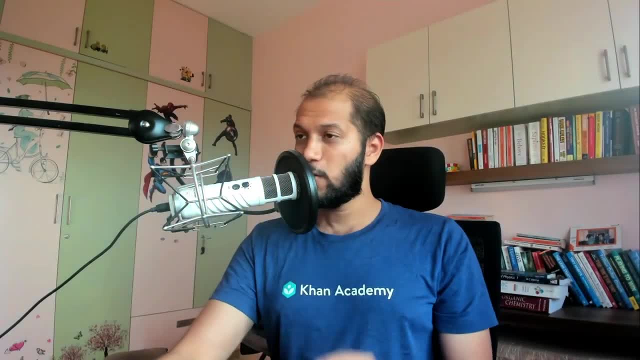 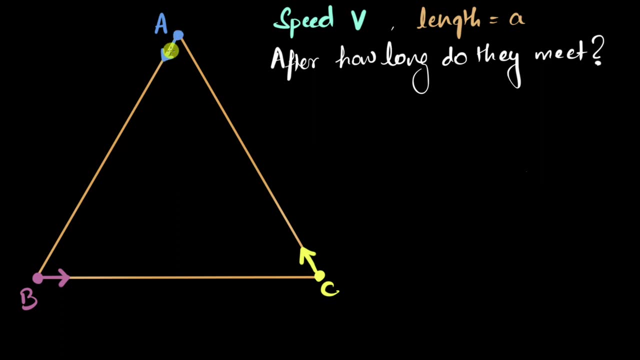 So here's how you tackle when things are continuously moving. You can assume you can take small time step and in that time you can assume that their velocity stays the same. So over here I can assume for a small time A's velocity vector is gonna be in this direction, B's velocity. 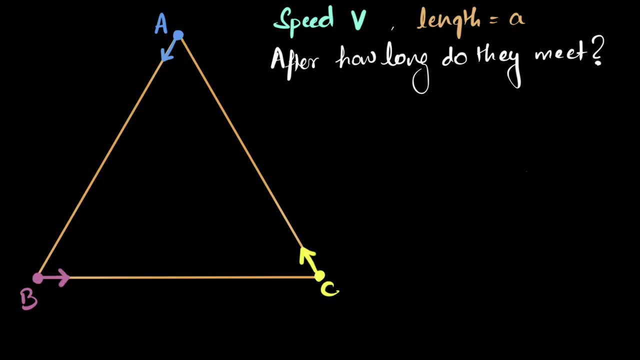 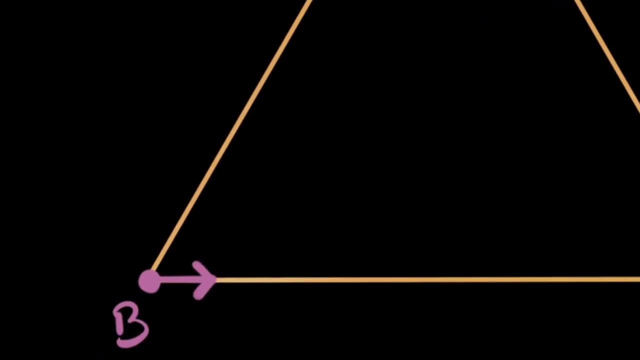 will stay in this direction and C's velocity will be in that direction, Which means in that small time A will come from here to here. B would have traveled the exact same distance here. C would have traveled the exact same distance here. 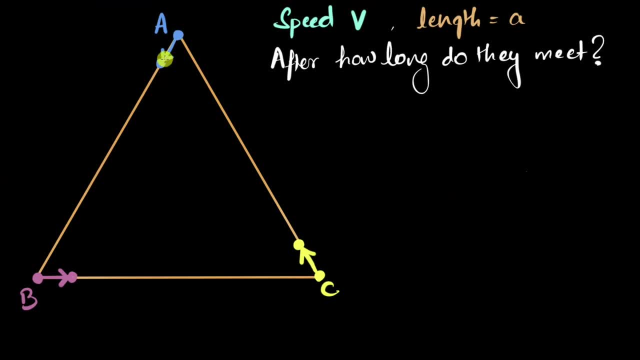 And now we can update their velocity. We can now say: aha, the new velocity of A is going to be towards B. It will have the same speed because of constant speed, but it'll move towards B, so it'll be pointing towards B. 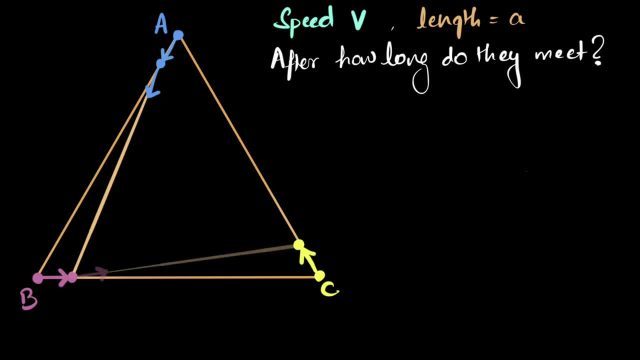 Similarly, B will again update its velocity. it's gonna be pointing towards C and C will be pointing towards A And we will repeat: We'll again wait for a small time interval. We'll assume the velocity is a constant in that time interval. 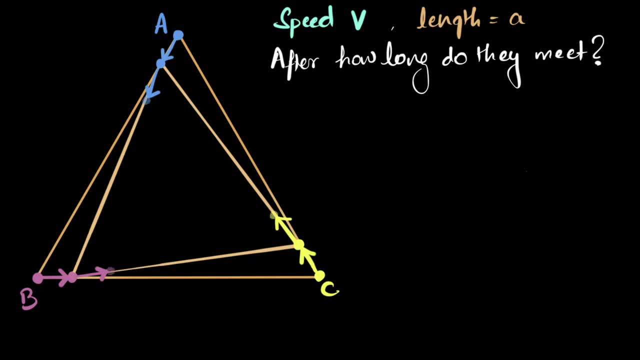 and that means your A would have traveled a little bit further, B would have traveled a little bit further, C would have traveled a little bit further, And we can keep on doing this. Now we'll update their velocities, which means A will be pointing towards B. 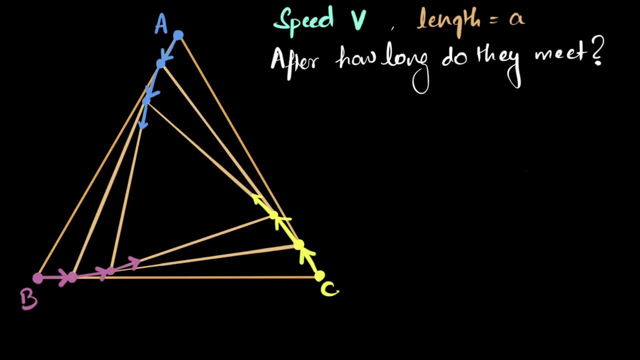 B will be pointing towards C, C will be pointing towards A, And we keep doing that again and again and we can now visualize their motion And you can kind of see, ah, they're now all going to go in a spiral. 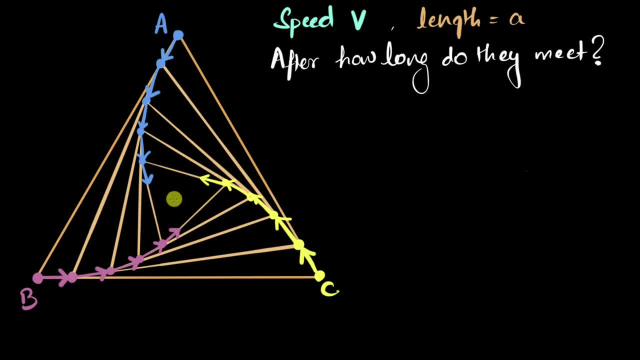 not a spiral, in a curve like this, and you can kind of sort of see that they're gonna meet somewhere at the center. Now this question makes sense. And if we were to look at what would actually be happening, because this velocity will be continuously changing. 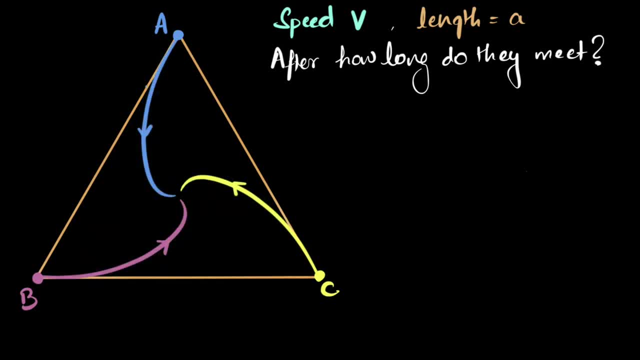 then the final picture would look somewhat like this: Now we have visualized the problem. Now we have visualized the problem So we can figure out how long it takes for them to all meet towards the center. Now, how do I do that? 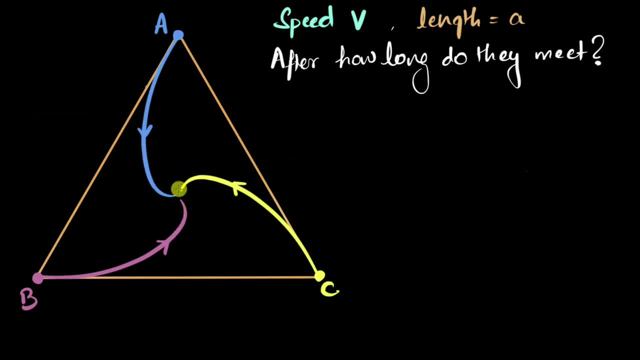 I know the speed- the speed is gonna be the same V- but I don't know the distance. This is a very weird curve distance. I don't know what that is. So how the hell am I supposed to find the time taken? 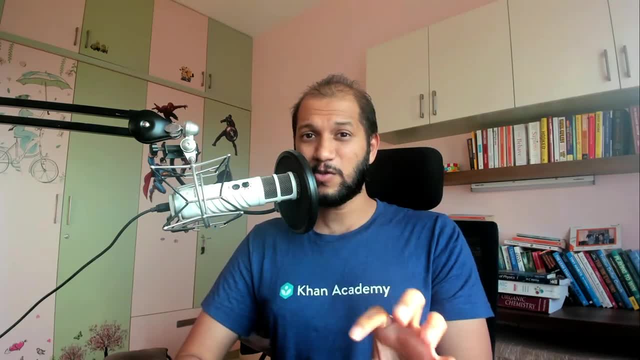 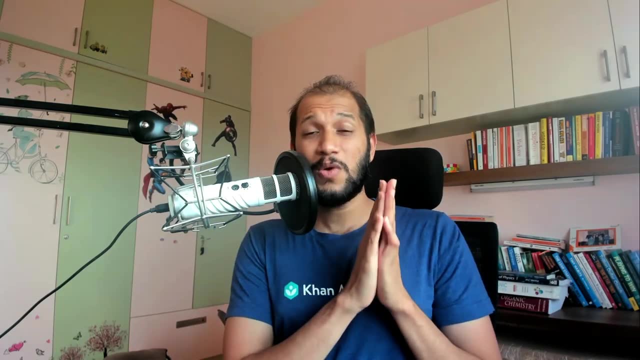 After spending a lot of time on this problem, I realized here's the secret to solving not just this problem, but all other problems like this: When you see that the most straightforward way doesn't give you the answer, you have to change your perspective. 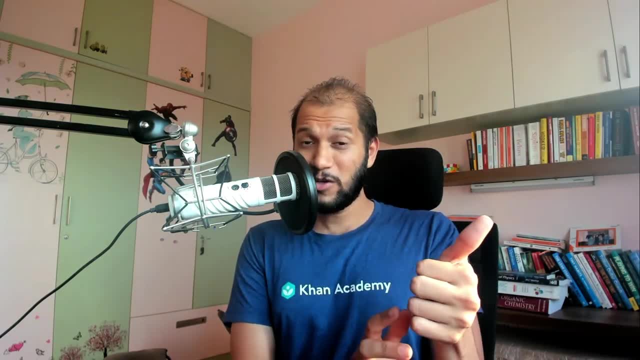 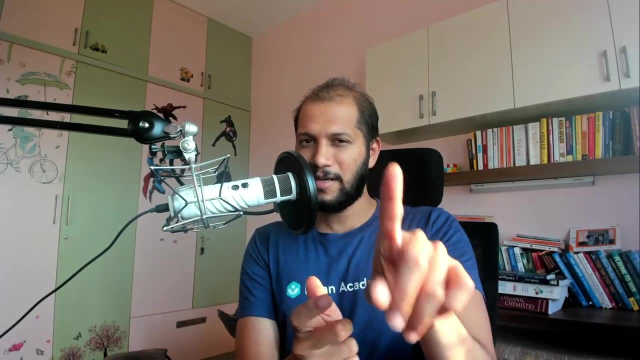 I know that sounds vague, but in physics it would mean a few things. One, it could mean you change your reference frames. Or another way to think about it is you change the problem statement a little bit. Here's what I mean. So our original problem asks us: 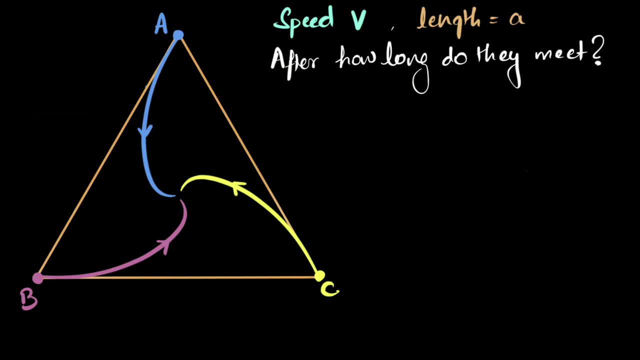 how long it takes for them to meet right. But if we go back to the kind of pictures that we drew, we can see something else. We can see that this original triangle that we began with the triangle starts becoming smaller and smaller. 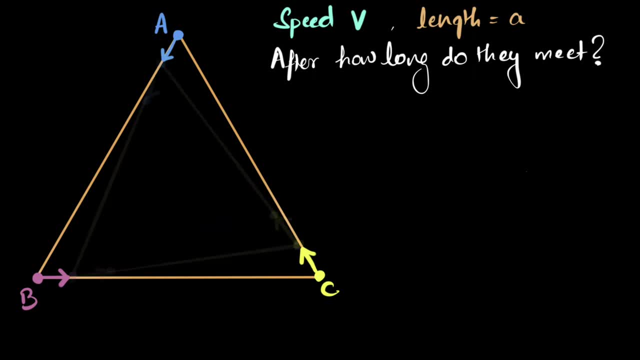 Let me show you. So you have this big triangle with length A to begin with. A little later in time, look, the triangle becomes smaller, becomes smaller, becomes smaller and smaller and smaller. So what do you think is gonna happen when they all meet? 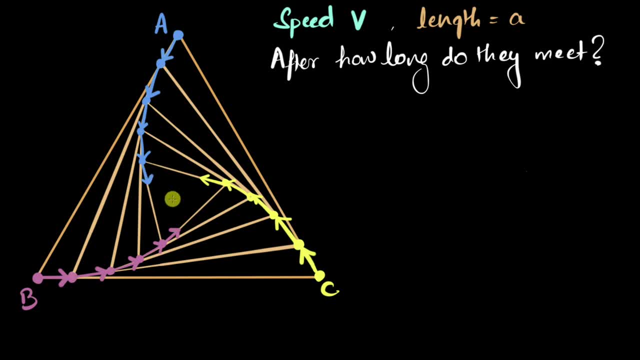 That triangle is going to vanish. That triangle's size is going to be zero. The length is going to be zero, Which means we can. another way to look at this question is we can ask: hey, how long does it take for the length of this triangle? 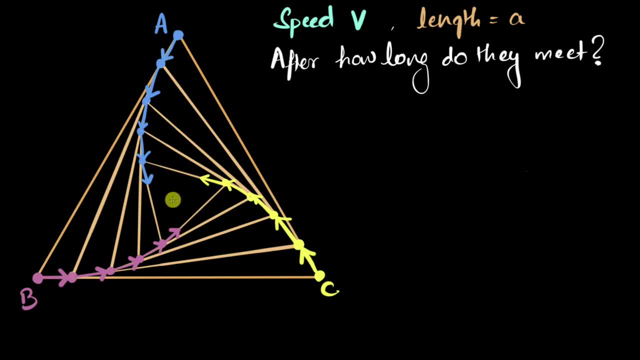 to go to zero. That's our new perspective. If we can figure that out, we're done, And it looks like we can kind of sort of do that. But how do you do that? Well, for that I'm asking myself. 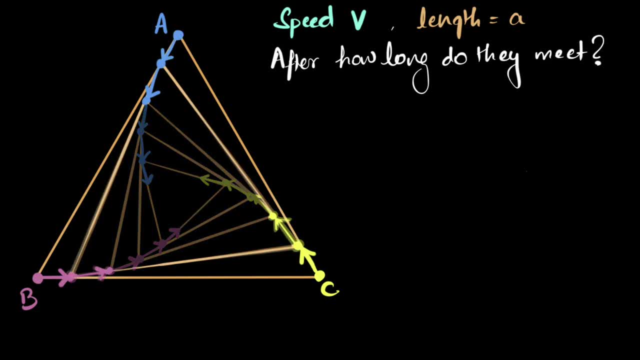 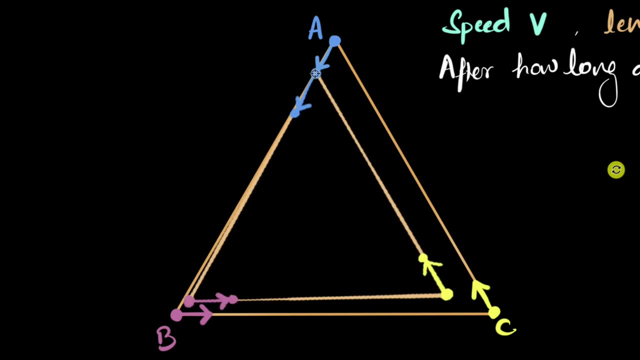 what's making the length of that triangle shrink? Let me get rid of the other triangles, And what I'll do now is I'll take this triangle and I will rotate it so that it's aligned with the bigger triangle And we can see the picture clearly. 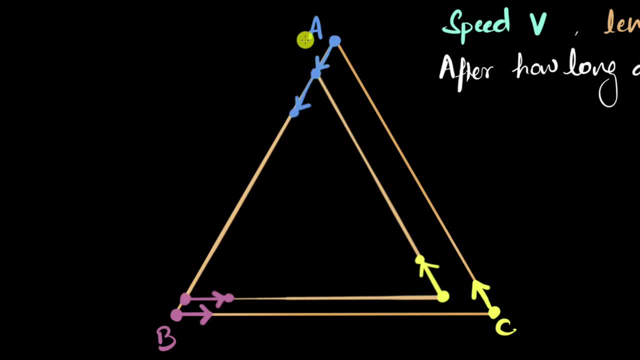 What's making the length shrink? Well, it's the fact that A is moving towards B, But it's not just that. You can also see it's shrinking from here. Somehow B also happens to be moving towards A. Why is that happening? 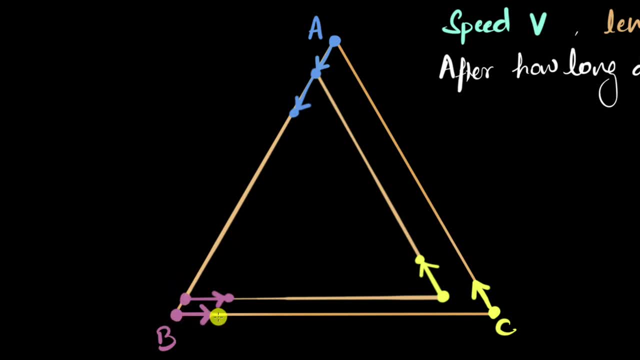 It's happening because, although B's velocity vector is towards C, that velocity has some component in the direction of that A And that component is making B also move towards A And if I draw another triangle, same picture- A is moving towards B. 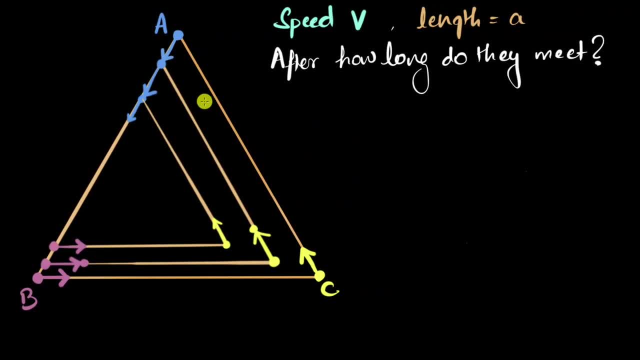 A is moving towards B. A is moving towards B with the velocity V, B is moving towards A with the component of the velocity in its direction, And these two, since they're moving towards each other, eventually when they meet? that's what we need to figure out. 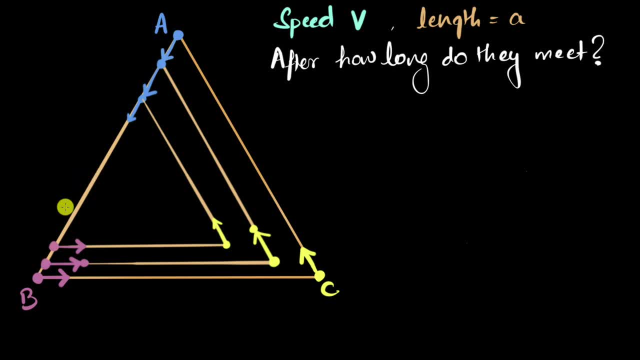 how long it takes for that to happen. In other words, all I need to do is figure out what their relative approach speed is. Think about it: They began with a separation of A and they end with a separation of zero, because they're gonna meet each other. 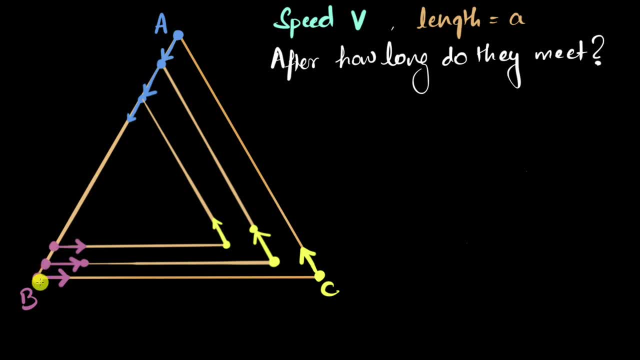 So I know the distance they're gonna travel. If I know, if I can figure out what the relative speed is, then I can figure out what the time it takes. Now would be a good time to pause the video, complete the dots and get the answer. 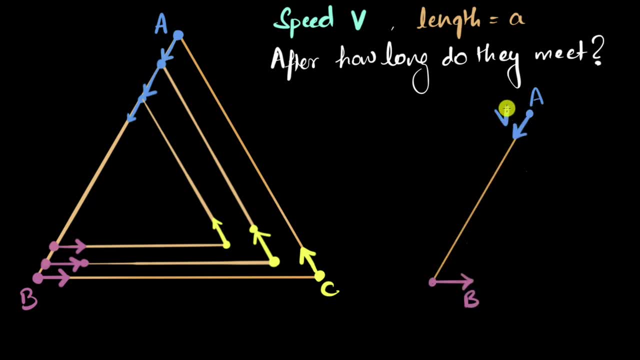 All right, let's look at it over here. I know A is traveling towards B with the speed V. B has a component in this direction And that component is going to be this. velocity is V, So that component is going to be V cos of this angle. 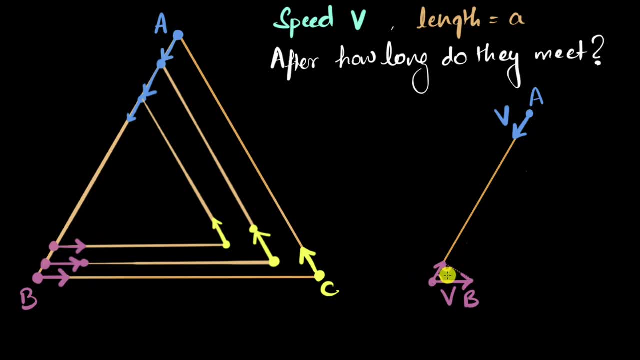 But what is this angle? Well, since it is equilateral triangle, that is 60 degrees. So this is going to be V cos 60 degrees, or that's going to be V divided by two. So B is approaching A with the speed V by two. 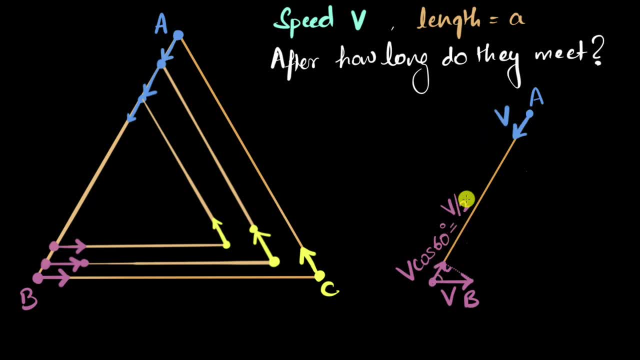 A is approaching B with the speed V, What's their relative speed? Since they're approaching each other, we can just add them and we can say the relative speed. I'll just call this V. relative is going to be V plus V by two, that's three, V by two. 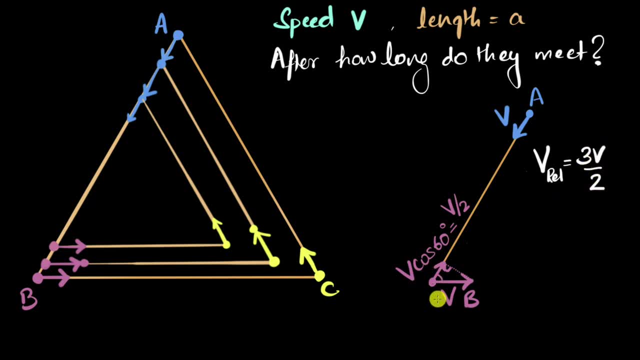 This is their relative approach. speed, which means if I look at from B's perspective, then everything appears. B appears to be at rest and A appears to be moving towards B along this direction with a speed three V by two. What is the relative distance that they're covering? 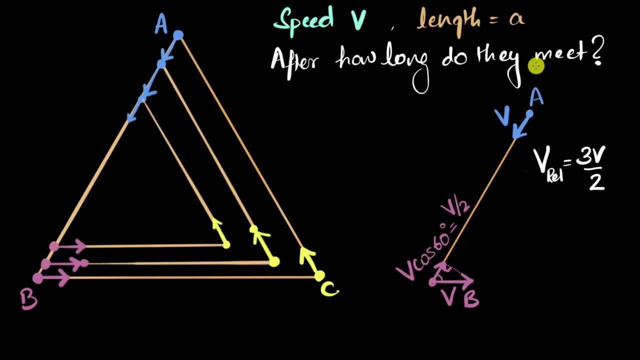 From B's perspective. A was at a distance A and B was at a distance B, So it's going to be A to begin with And then at the end of time it has come and met. So the distance that they have traveled relatively is: